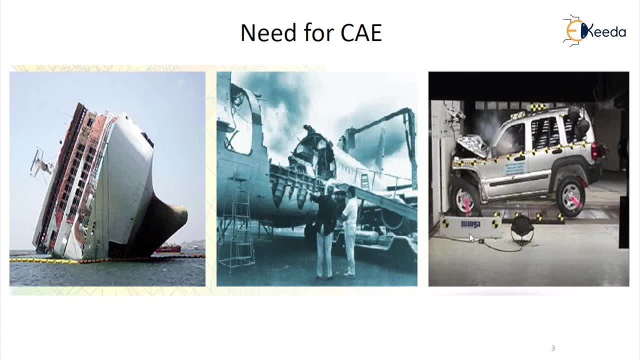 awareness of issues such as safety, economy and environmental sensitivity, so that these issues will be required to solve by using computer aided engineering. So it is one of the proven technologies which is used to solve these issues. So it is a need of a. C is to design, manufacture. 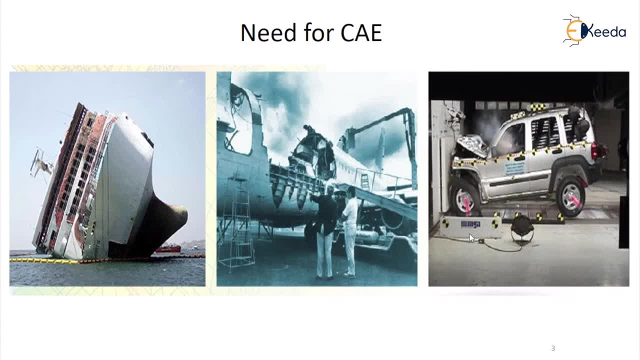 operation and maintenance of a safe and reliable engineering product has become increasingly important today, Which has in designing efficient and failure safe products. So first usually indicates the treating of a ship due to some of the not properly covered or not properly. We have to manage those condition. So due to that, a ship is treated Sometimes. 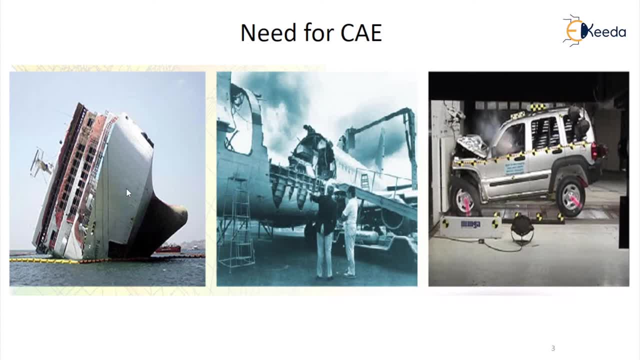 we are going through the why the aeroplane crashed or why the design was not done properly, why the aeroplane having some of the different disasters happened. So what is the main cause? We need to find those things with using CAE and, lastly, that vehicle worthiness or 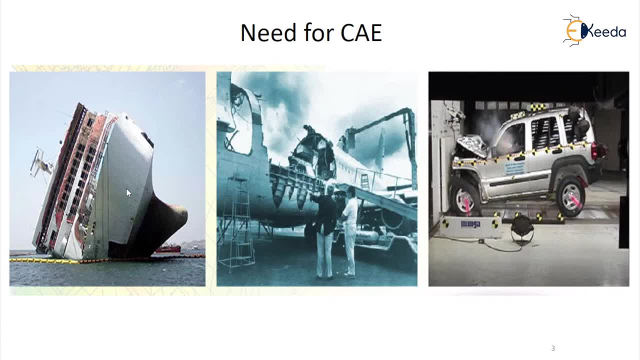 cash worthiness of the any type of four-wheeler. So we can here observe the exact position or how whether the our airbags are working properly or not. So need of for CAE or need for FAA is very important nowadays or every time for doing the analysis of different kinds of conditions. 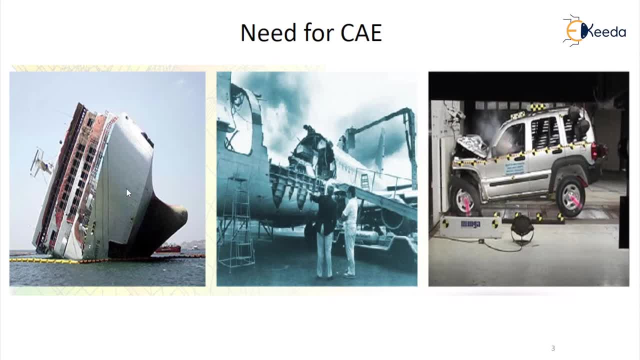 So these things are very important because if the small component analysis is not taken properly, it will fail the entire machine or entire product, and that will happen. natural disasters, So we have to reduce those disasters due to humans where the human loss will be taken place. So those we need to be reduced by using CAE. 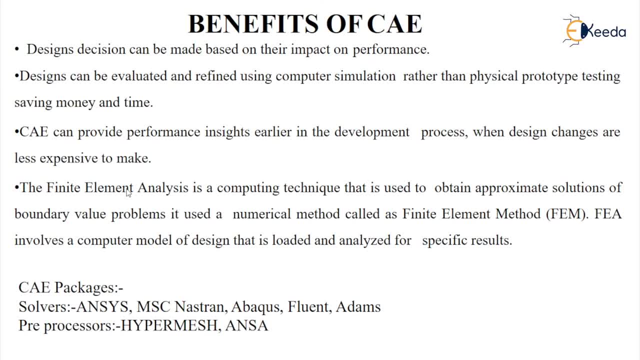 So benefits of CAE. if you observe that design decisions can be made based around their impact of the performance, Designs can be evaluated, redefined using computer simulation Rather than physical prototype testing, saving money and time. So instead of making a prototype, we can easily save the time and money- Then CAE can provide performance insights. 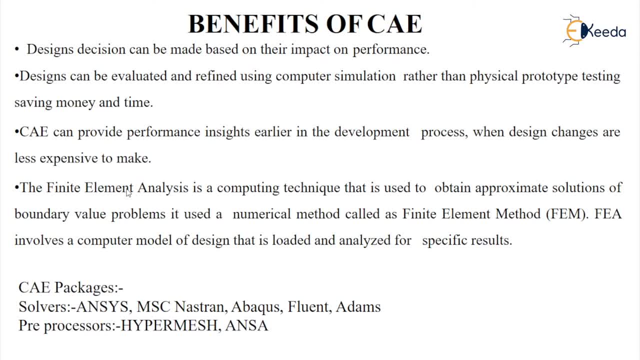 earlier in the development process when design changes are less expensive to make, And the finite element analysis is a computing technique that is used to obtain approximate solutions of boundary value problems. It is used in numerical methods that is called a finite element analysis. CAE involves computer model of a design that is loaded and analyzed for specific users. 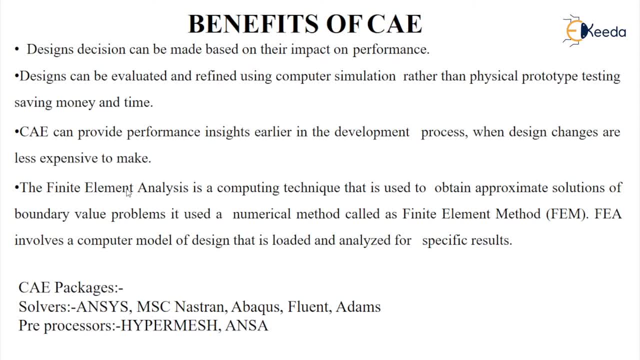 So some of the benefits. also, it reduces the physical testing and saving money. Innovate faster and beat your competition. Keep material cost in check. Then tick design before production. These are the very most important parameters of benefits of a CAE. So CAE packages are answers now. 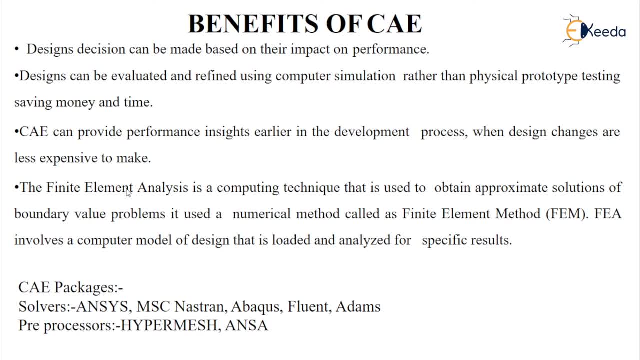 SAPTAN, SATRAN, ABACUS, FLUENT ADAMS, SERVICE, SEVIR SOLVERS are available And preprocessor, HyperMesh, ANSSTAR Compound Sciences model also. we can use HyperMesh also having some of the solvers like RADIO TOPSYSTEP for solving the different types of problems of computer RAID. 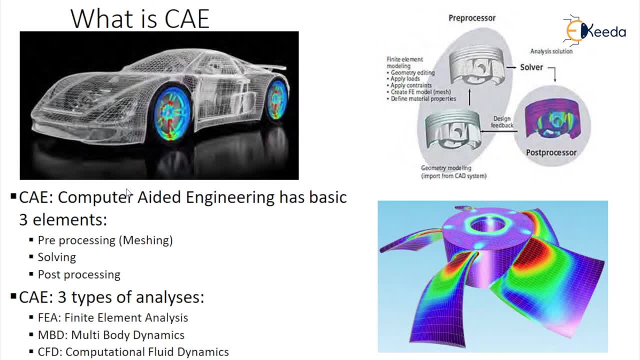 Then what is CAE? Computer Aided Engineering is a broad range of computers, software in aid, in the finite element or in engineering analysis class. it includes the finite element analysis, then computational fluid dynamics, multi-body dynamics and optimization. yes, it is considered in computer-aided engineering, computer-aided engineering. 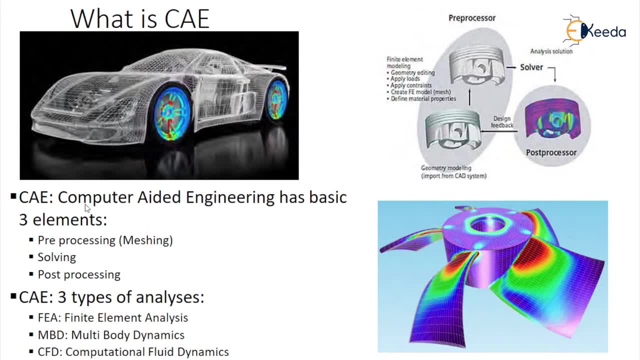 having three main parts, that is, pre-processing, solving and code processing in pre-process. or, if you observe there is only geometry or modeling. by using any type of cat software like patria, ugns or any type of oe trio like this, you can design or you can create a geometric model. 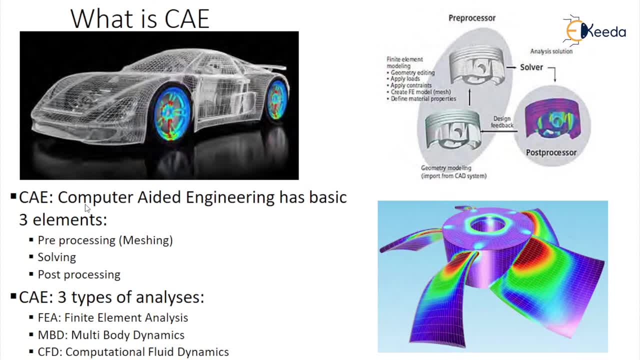 then in pre-processor we have to define or create a finite element model. that means we have to create a model with a different discrete part. so while discretizing the part is shown in this car model, that is, every part is having meshed like structure. that means every. 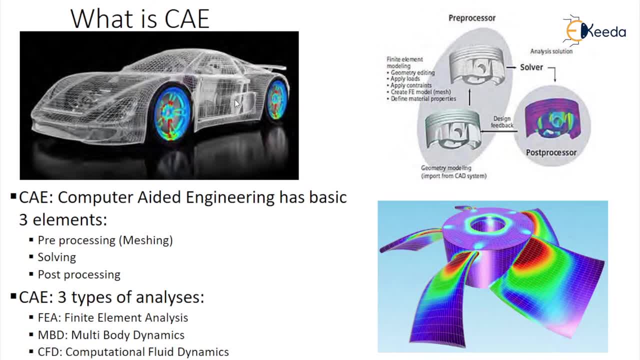 part is having small, small elements, sometimes the angular, sometimes the square, as shown in this figure, so those are need to be understand. there are nodes and elements, so geometry editing will be there. applying the loads will be there. applying the constraints will be there. creation of the finite element model will be there for meshing and define. 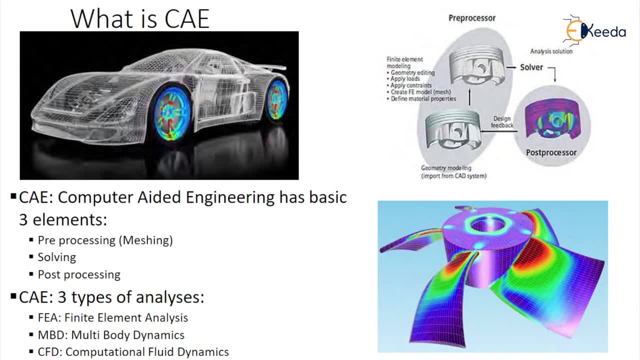 material properties. those are very important in pre-processor. then there is a solver, that is analysis solution, where the analysis solution- that means calculation part- will be started when we run the program. we run the. after applying those condition, we run the process or procedure like static analysis, dynamic or dynamic analysis. it was called by different methods at the back end and 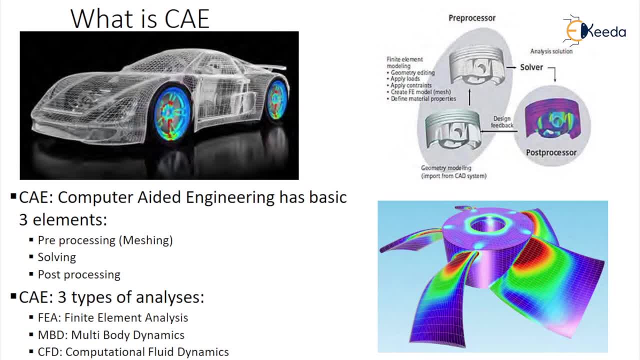 at the post-processor you will observe the actual the structure, with having a different areas where the stress concentration is maximum. okay, so like this, you will observe there is a green zone, red zone, orange zone and the blue zone. blue zone having very less stress, where red zone having very. 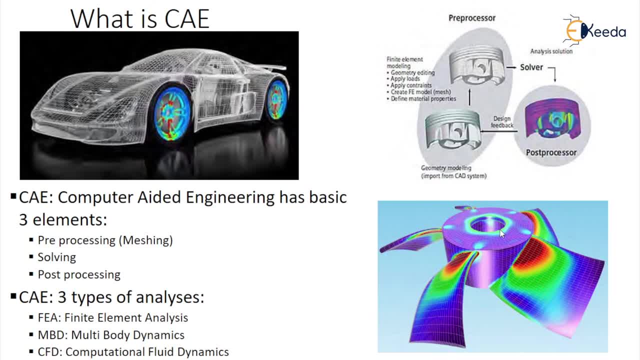 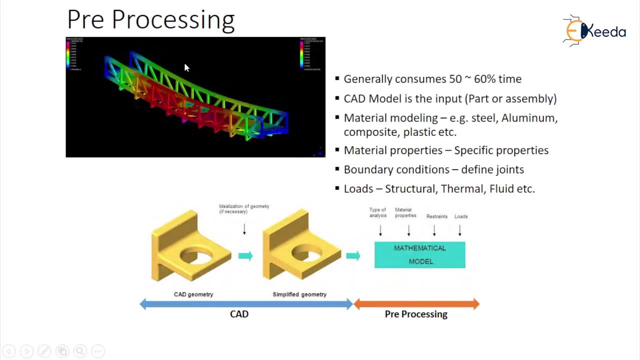 maximum stress, so where the breakage and where the maximum stress will be occurred at the red zone. so that is very important, important part of CA. similarly, here also you will visible, for cantilever or simply supported fridge, pre-processing will be taken plus pre-processing, then CAD geometry making, idealization. 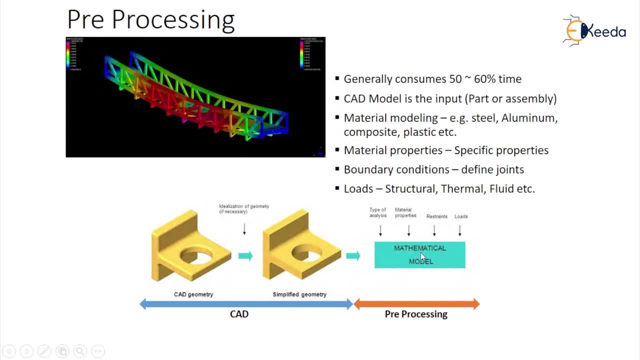 of geometry and simplified geometry, then mathematical modeling. that is type of analysis. material properties, restraints and loads are applied. so generally it consumes 60 to 60 percent of time. CAD model is a input that is part or assembly. sometimes it is part, sometimes it is assembly. material modeling, for example, feel, aluminum, composite plastic. we have to 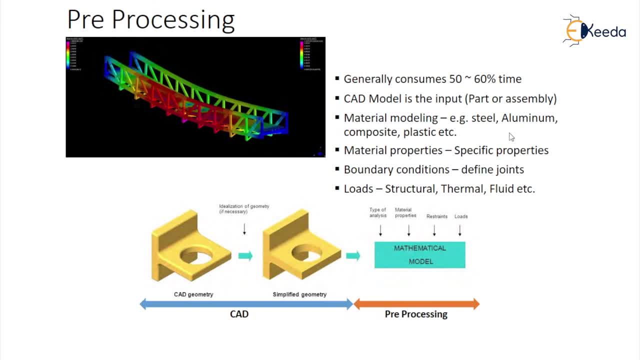 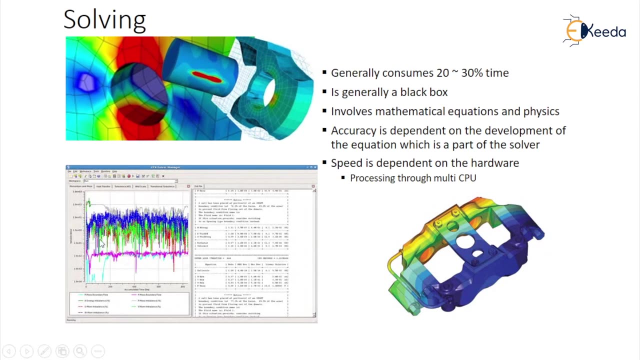 give material property. so we have to specify the property and boundary conditions to define the joint and load, our structural thermal fluid load. these are etc. solving. so in solving, if you observe this follower is there at the back end how it is- a computational will be taken place where we are. 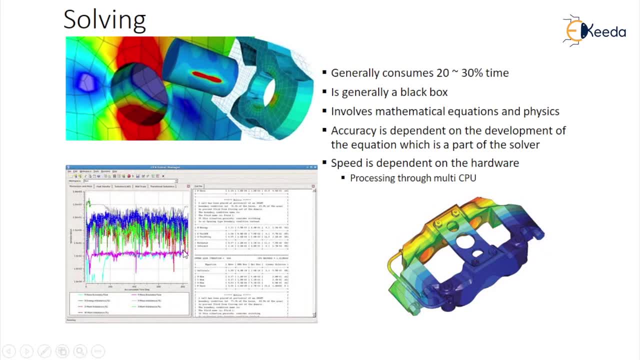 getting a conversion of tweezers. so that's where, as you see, if you have to start with the actual, So that time it will be stopped. So these are the nothingness solving Generally it's under 20 or 30 percent of time and it's generally a black box and involves. 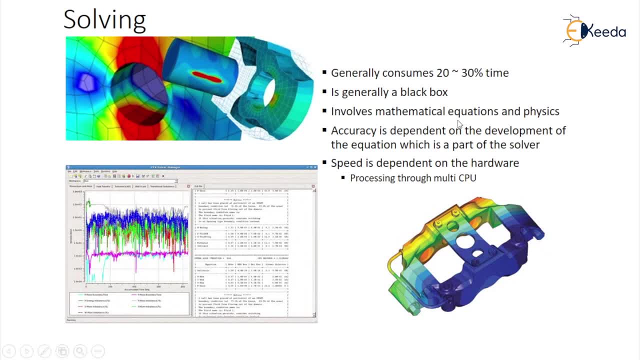 mathematical equations and fidget. accuracy is dependent on the development of the equation, which is a part of the solver. The speed is dependent on the hardware of processing through multi CPUs, So you can attach multi CPUs also and multiple RAMs of 16 sources you can use. 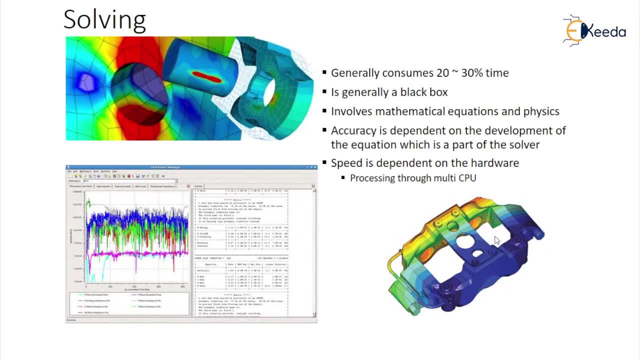 It depends on the time of solving, on how much RAM you have in the computer. So here also you will observe the different zones of area where the maximum rate having a maximum speed, and sometimes you observe the green and blue screen. So those are. 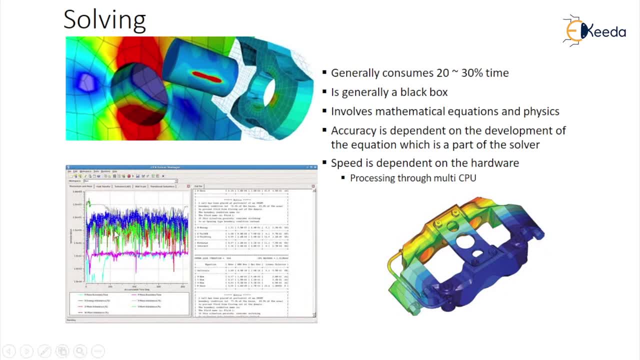 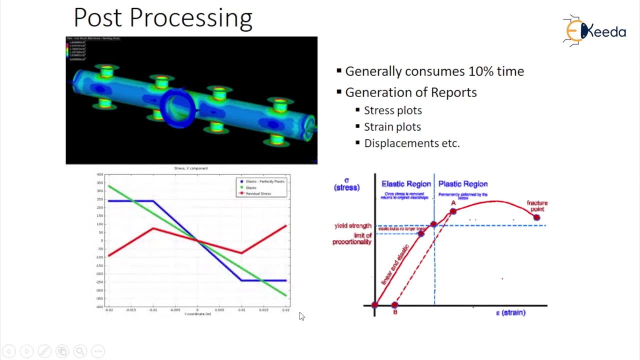 Here you observe, different types of computational will taken place at the back end side, So we can plot the graph also. So for post processing we are plotting the graph as shown in red, then red line, then blue line, and there are some blue lines we can specify. 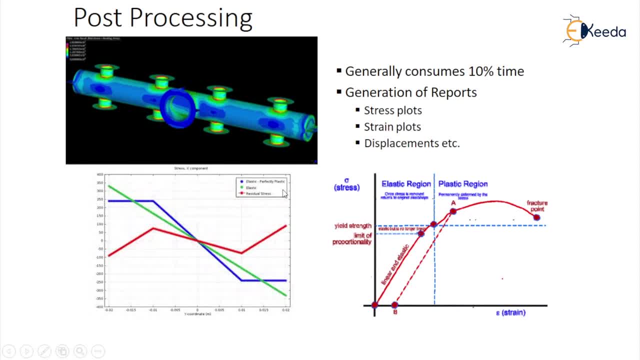 So blue line here specify elastic plastic material condition. Plastic condition will show by using a green line and residual stress will be shown by red line. So this is basically used. we are using a stress-strain curve. So according to stress-strain curve we are having elastic region. so at those region 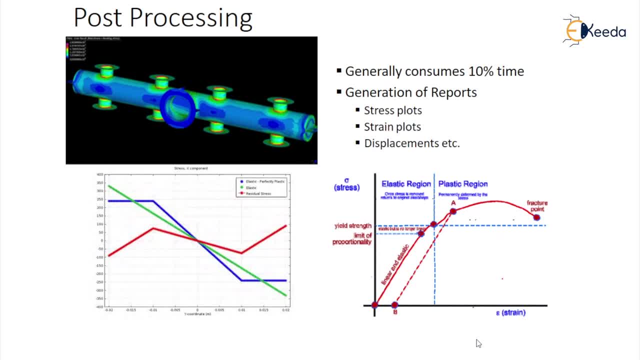 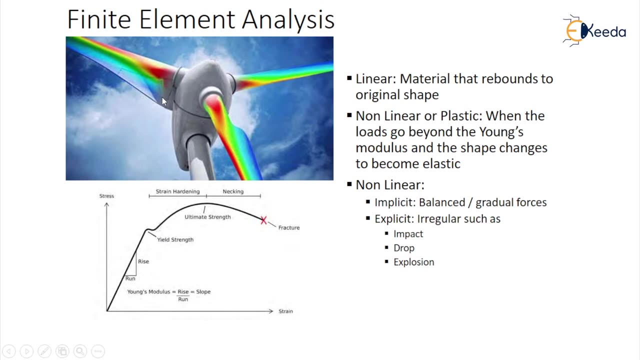 we will get the plot and it will consume only 10 percent time. After solution, the post-processing takes place where the different plot or these graphs and these animations. So this is what we are going to do in the post-processing: Finite element analysis. 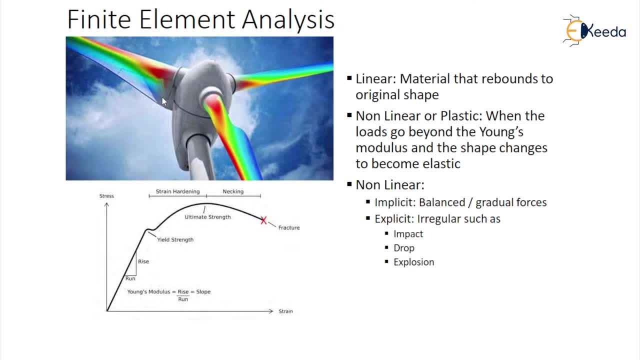 There are different types of linear analysis. non-linear analysis are there. Linear, that is restricted to stress-strain curve, that is elastic condition, So the material that rebounds to original shape. and non-linear, or plastic, when the loads are go beyond the nth modulus and shape changes to be become elastic. 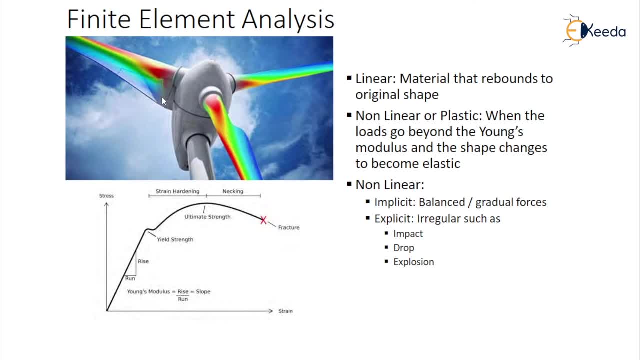 Non-linear condition will be done after the plastic region is start, elastic after plastic region will start. So implicit analysis will be taken first, that is, the gradual forces are applied that time, and explicit analysis taken first whenever irregular, such as impact analysis or impact. 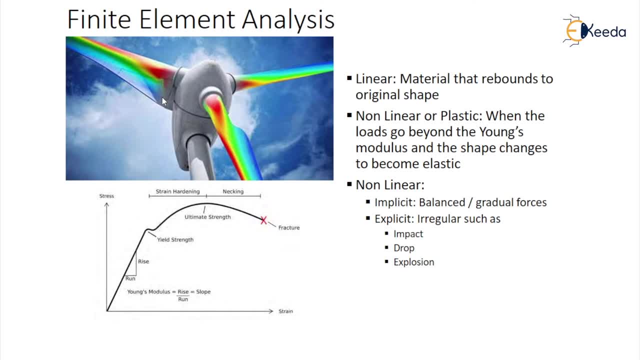 of a car, drop of any ball on the car sheath or car glass, then explosion. or sometimes we are using turning of a machine machining operation in balanced or gradual forces. So remember this non-linearity that is shown in this graph of the elastic region and plastic. 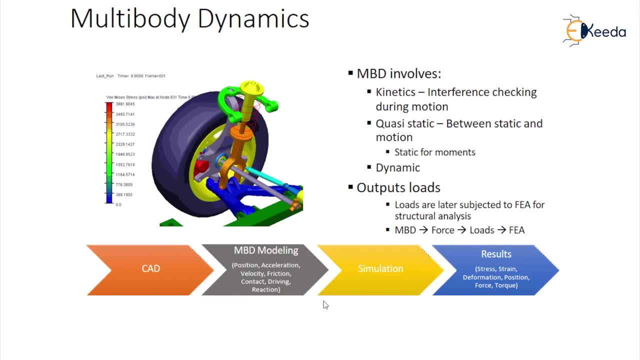 region. Accordingly, the analysis will be carried out Then multi-body dynamics, that is, kinetics, is involved here, Interference shaking during the motion. So there are multiple components are associated. So there are multiple components are associated. So there are multiple components are associated. 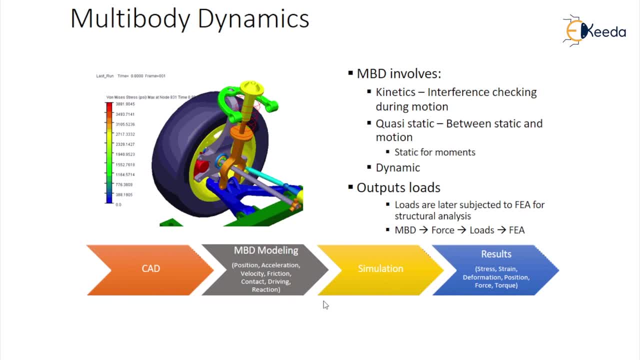 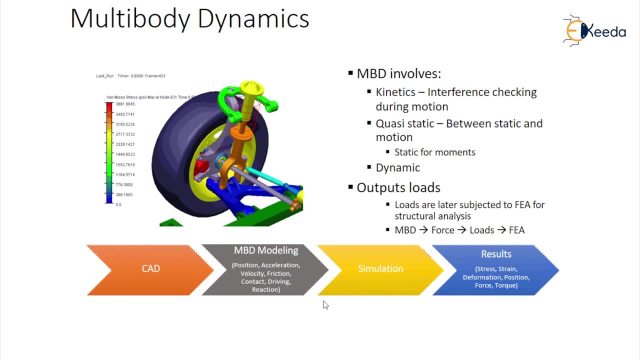 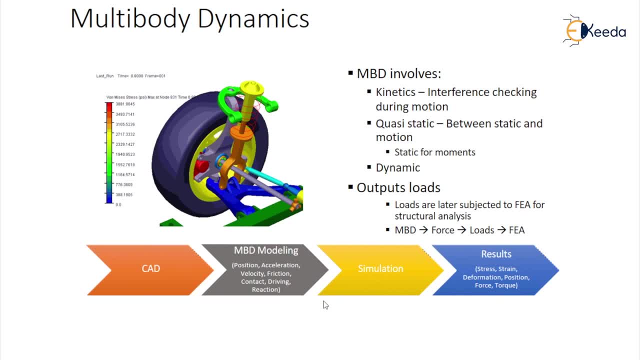 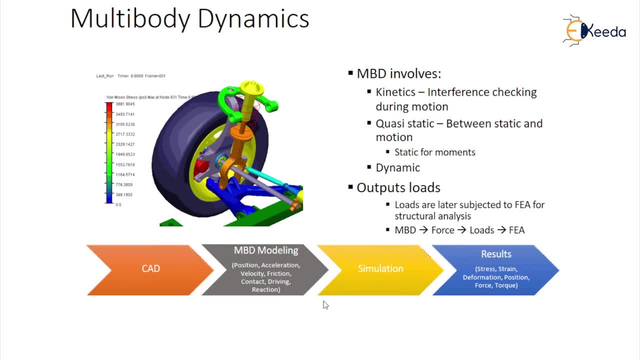 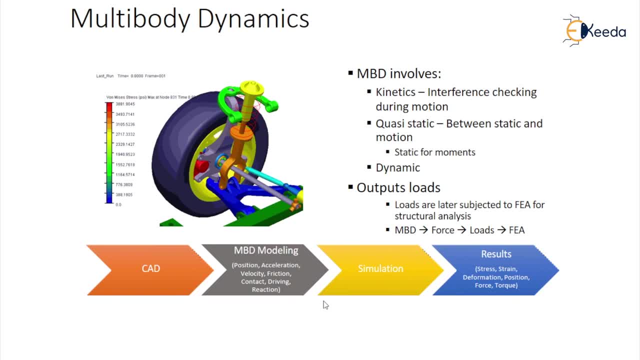 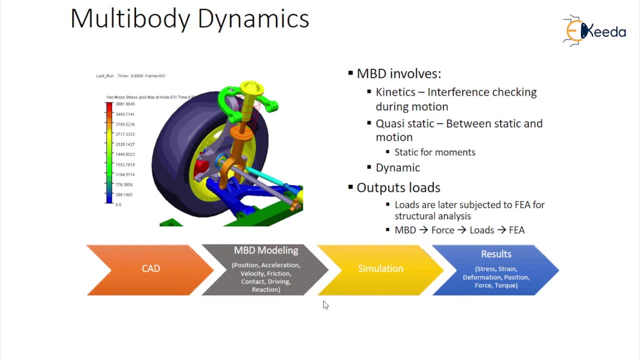 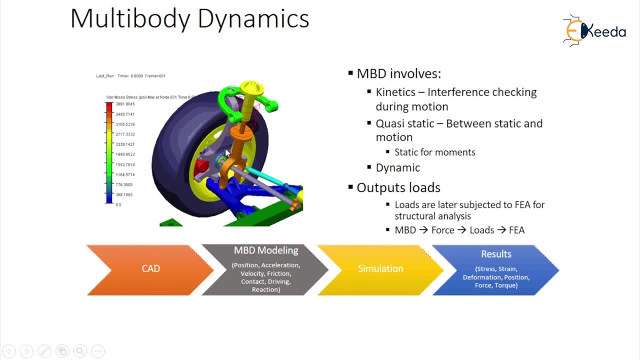 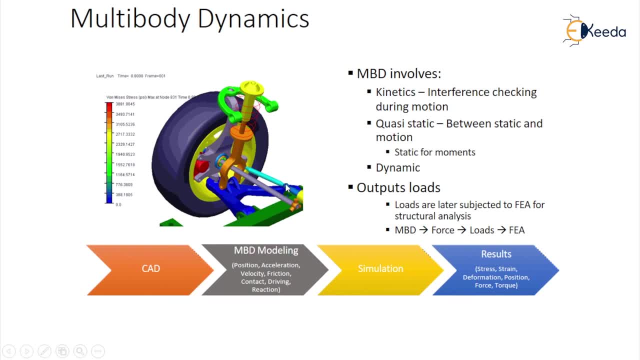